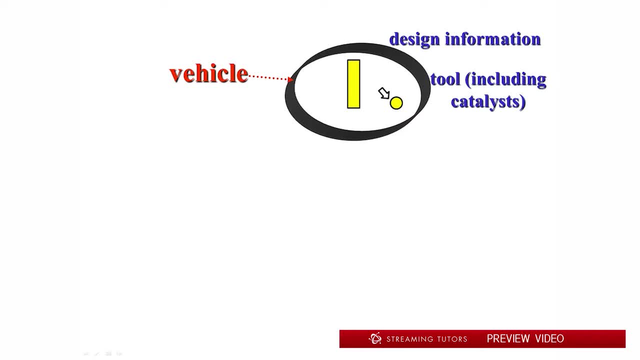 So remember that organisms- cheetahs or mushrooms or bacteria- are vehicles built by design information, behaving as if their goal is to replicate that design information, And in the course of doing that, they make a whole set of sophisticated molecular tools, including complex catalysts, that are encoded by genetic design information. 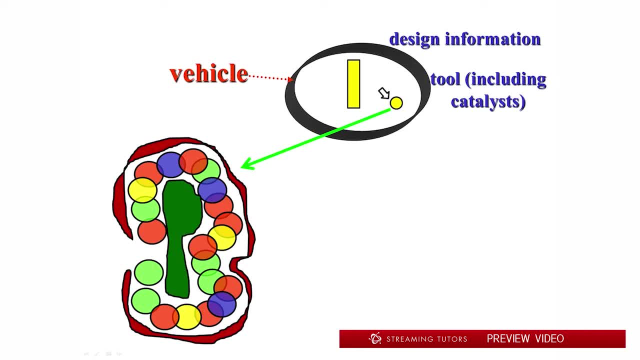 We've been spending a lot of time in the last several segments looking at the properties of those catalysts. We're now going to turn attention to some of the things those catalysts build And, in particular, macromolecular things those catalysts build. We're ultimately, in the next two segments, going to culminate with these large structures that define the boundaries of cells, membranes and so on. They are made of lipids. 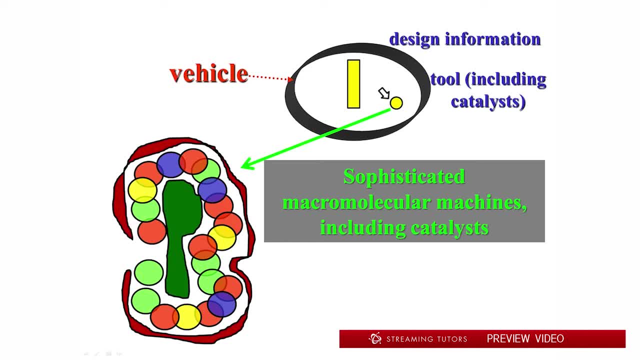 Our goal today is to understand the specific components of those lipids that are built by genetically encoded macromolecular machines. So let's be clear: We have genetically encoded protein macromolecular machines that then go on to build other macromolecular machines. 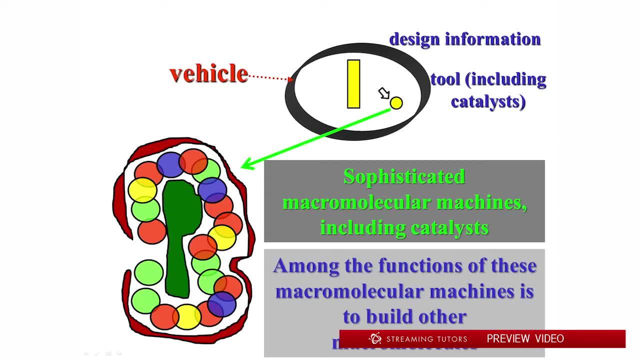 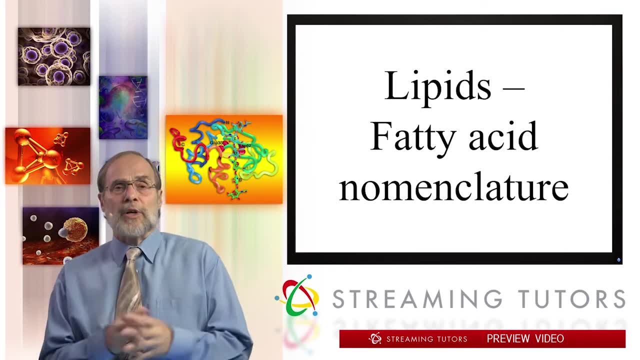 Some of which are built of lipids, And it's lipids that we're going to be focused on today. So let's focus on the sort of nomenclature and phylogeny, if you will, of lipid molecules That will be our focus in this segment. 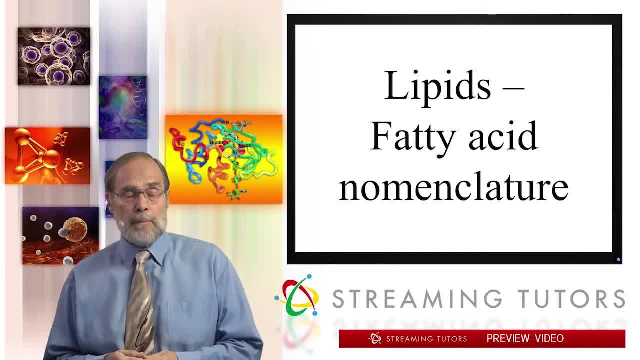 So we understand who the players are, who the actors are. At first glance, the phylogeny of lipid components, of larger structures like membranes, can be a little bewildering. There are several different kinds. Their structures at first glance look rather wildly different. 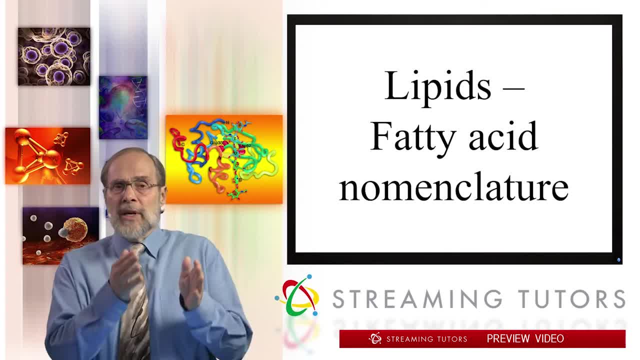 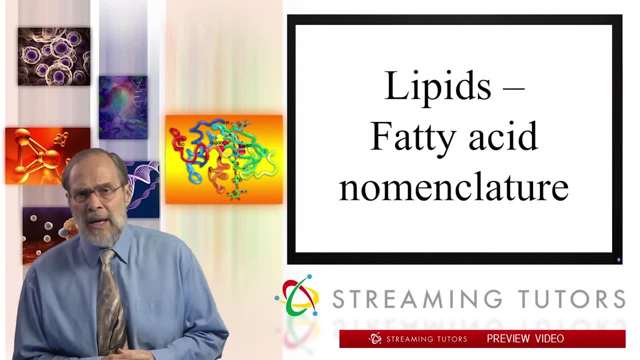 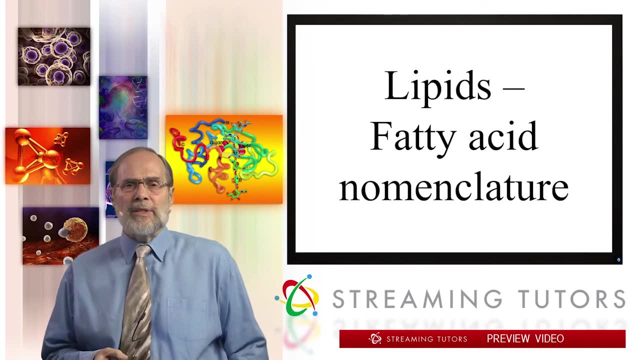 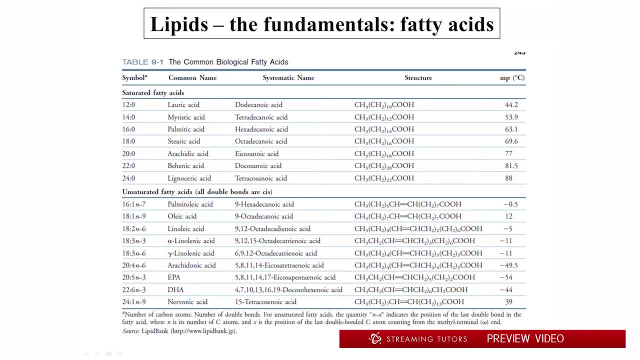 And that foolproof argument is really important. It's one of the reasons why you guys are going to notice. and diabetes, I sat study for stones fat fat kun fatun, with 12 carbons has a melting point above human body temperature 42 degrees centigrade human body temperature. recall is 37 degrees. 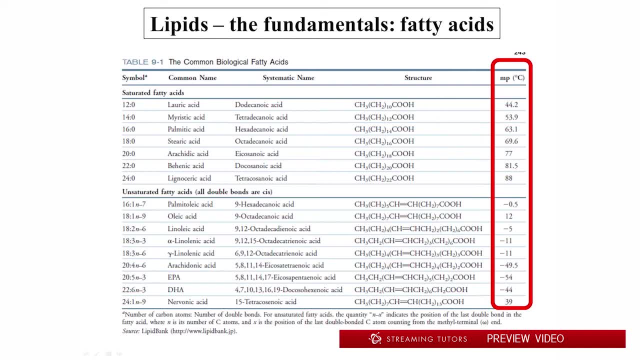 centigrade. and as these fatty acids get longer, their melting temperature gets higher and higher and higher. so these are solid. these would be solid fats at body temperature. in contrast, you look at the bottom half of the monounsaturated fatty acids. these monounsaturated fatty acids have much lower melting. 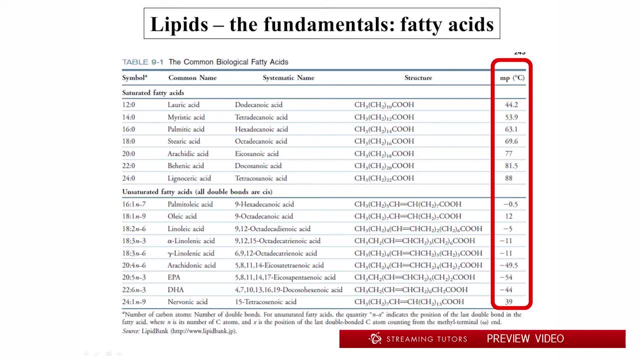 temperatures. all of them, with the possible exception of the longest one at 24, are well below human body temperature. so in some cases- I'm sorry, in some cases- they are polyunsaturated. you'll notice in the polyunsaturated ones have even lower melting temperatures. so let's now look at why that's. why that is the case. 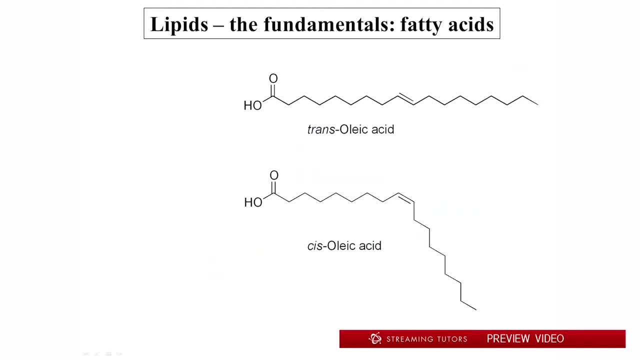 let's take a simple example. this is oleic acid, a common fatty acid in animals, and let's compare the trans configuration here, which is what is not built by biological organism. so we haven't said so yet, but the double bonds in fatty acids of biological lipids are almost always not trans. they 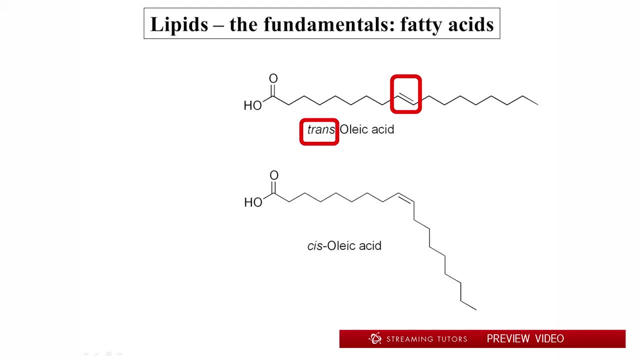 are cis. so let's look at the trans non biological configuration first. when the fatty acids side chain comes into a double bond on one side and then comes out on the opposite side, it has the effect of preserving the linear structure of that alkane side chain. on the other hand. 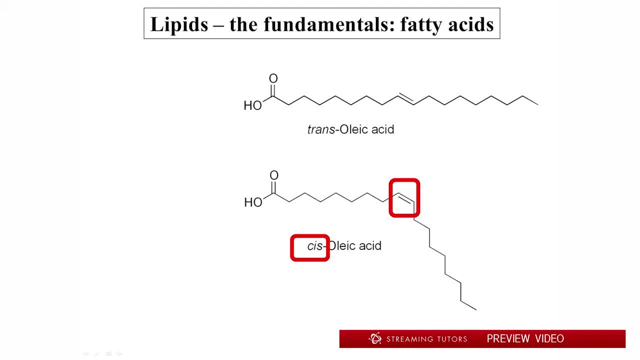 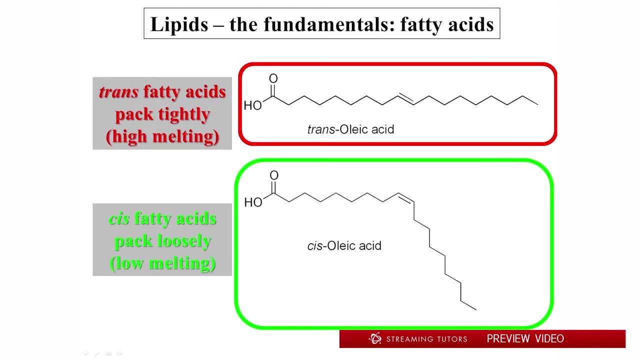 in the cis configuration. when you, when the alkane chain comes in one side of the double bond upstream and leaves on the same side downstream, the cis configuration has the effect of kinking the side chain. that's a huge difference. the linear side chains can pack together quite tightly with forming strong 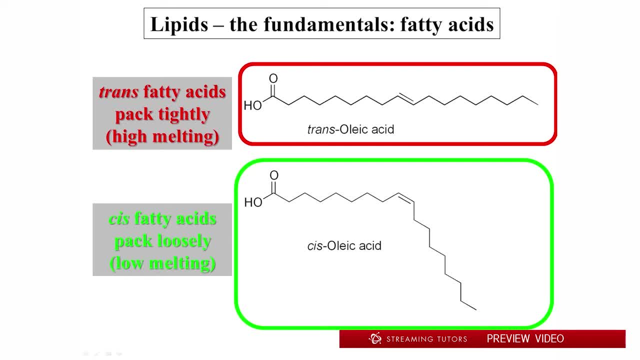 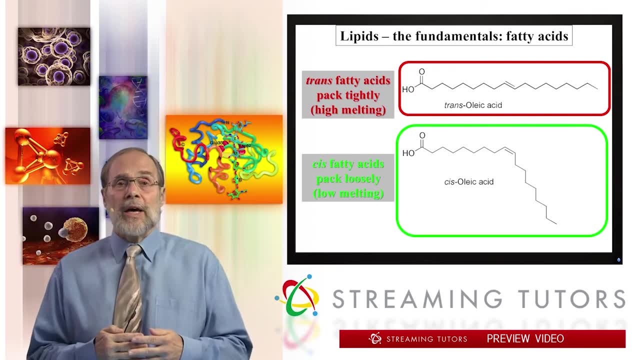 Van der Walls interactions and various kinds of hydrophobic interactions that we talked about so previously, and they tend to be high melting, the using, the use of cis fatty acids in fatty acids, an and biological membranes. these kinked fatty acids, those fatty acids don't pack together. 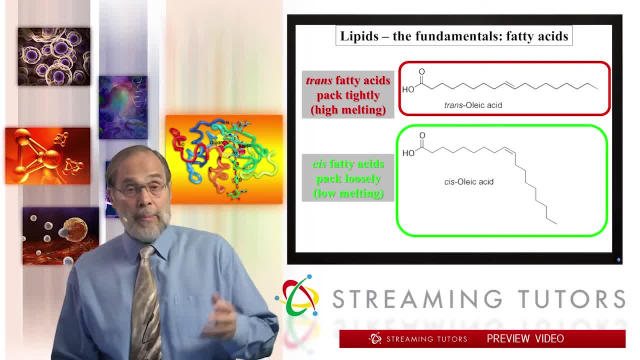 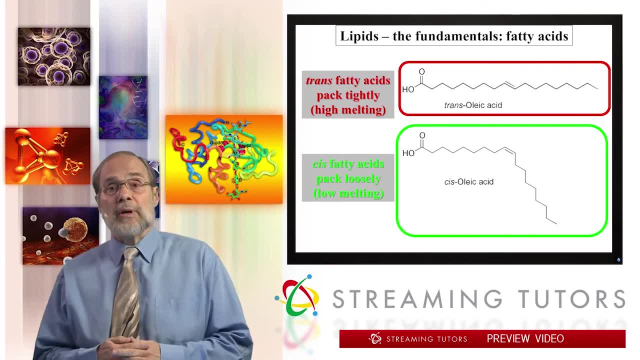 as efficiently and they melt at much lower temperatures. So, as you might imagine, biological organisms are going to control the relative amounts of both saturated and unsaturated fatty acids. and because the unsaturated fatty acids are cis, by adding unsaturated fatty acids to the membrane lipids, you're going to reduce its melting temperature. You're. 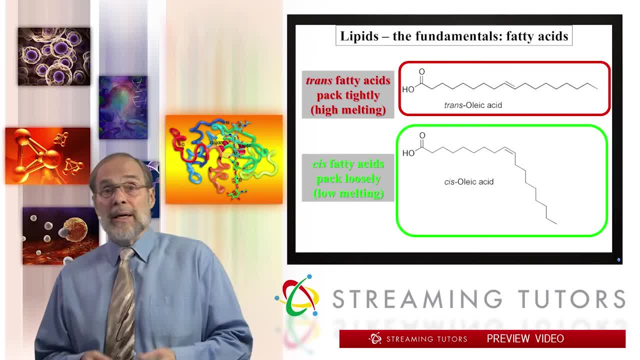 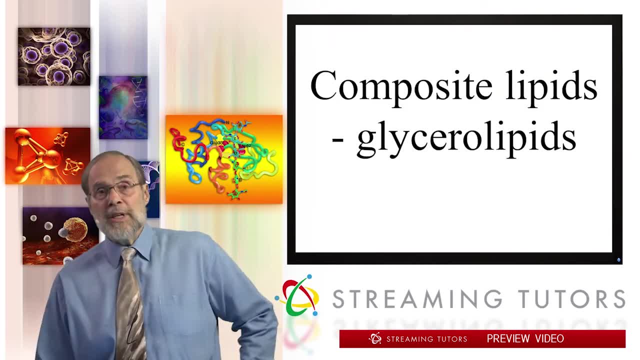 going to control its fluidity, how much it's like an oil and how much it's like a solid fat- again a subject we'll come to in the next topic in more detail. Alright, so let's now start looking at how these fatty acids get combined with other components to make 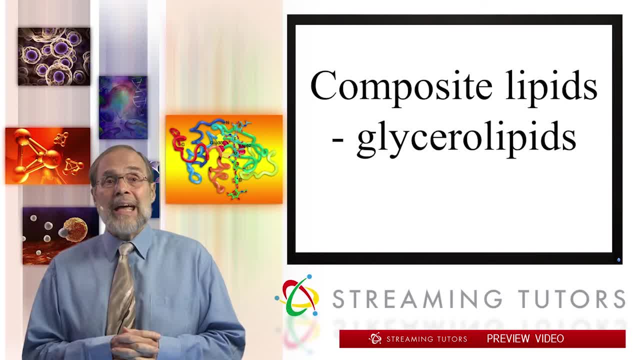 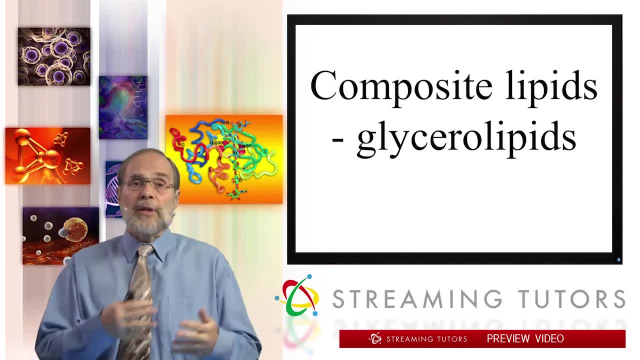 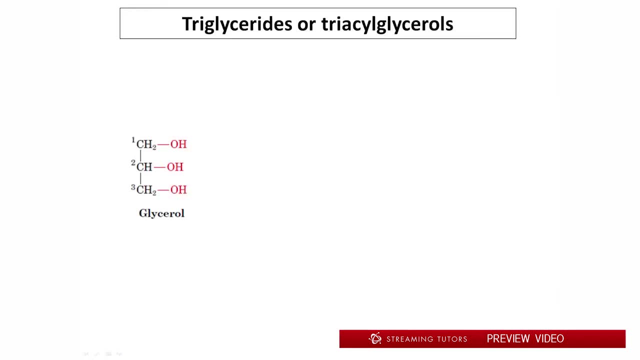 the actual larger subunits that make up biological membranes and lipid-based biological structures. We'll call these composite lipids, because we're putting together fatty acids and other components to build the actual unit that's going to be assembled into a membrane or whatever else. it might be A very large class of these composite lipids. 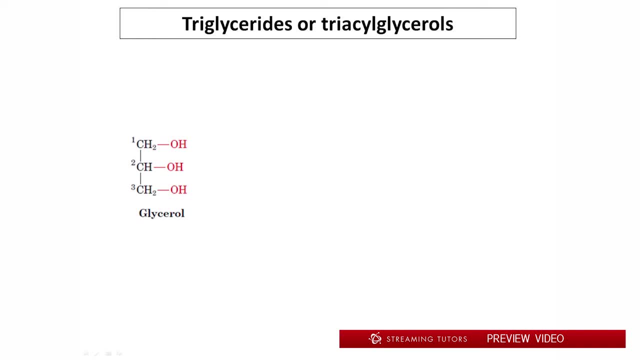 are called subunits. Subunits are built around the 3-carbon glycerol skeleton shown here. Remember, glycerol has three hydroxyl groups. It's an alcohol with three groups on it, And when fatty acids are bound to all three of those groups in ester linkages, you have what's called a triacylglycerol. 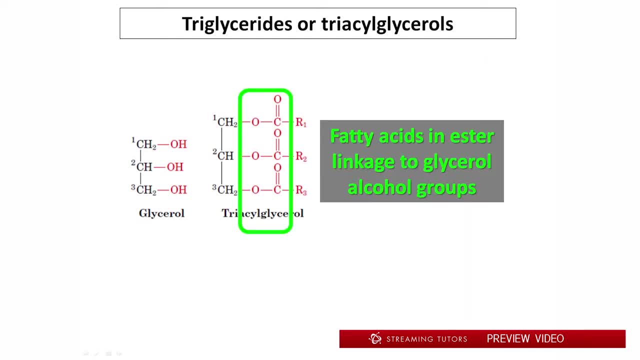 Now, what I want you to notice here are two things. If you look at the fatty acid- let's go back to that image- if you look at the fatty acids bound here, they're bound in ester linkage to the hydroxyl groups of glycerol. 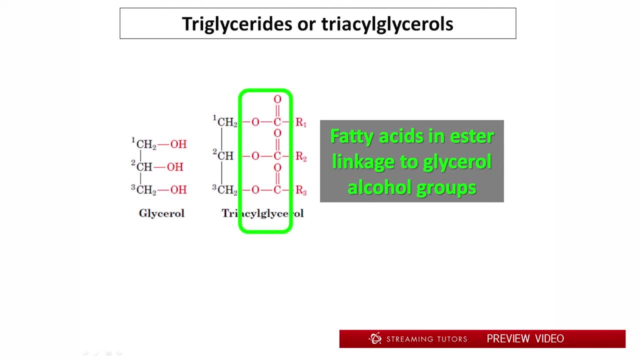 And as a result, there's no charge, right? The fatty acid acyl group is not ionized now. it's bonded in a neutral ester linkage. So when you make a large triacylglycerol in this way, you're making a neutral lipid. So neutral lipids are, in fact, very hydrophobic, Even.